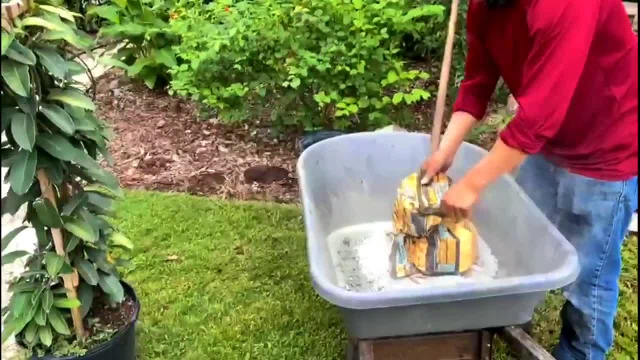 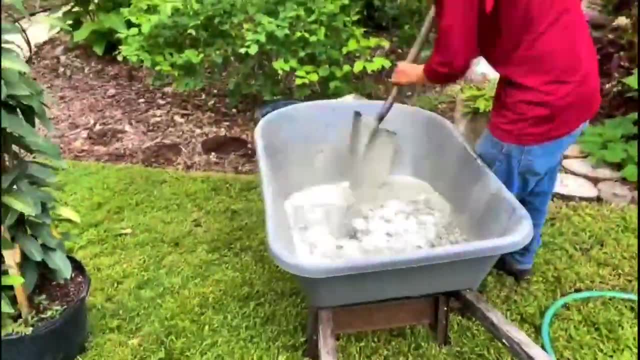 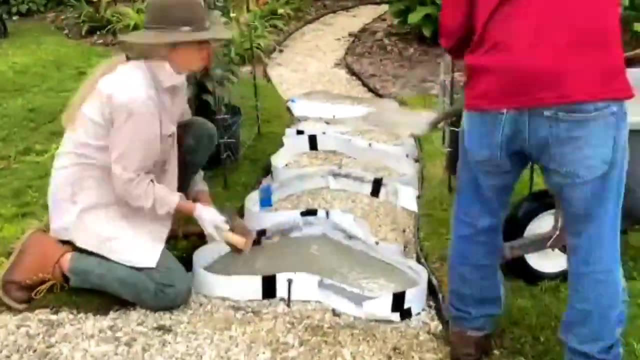 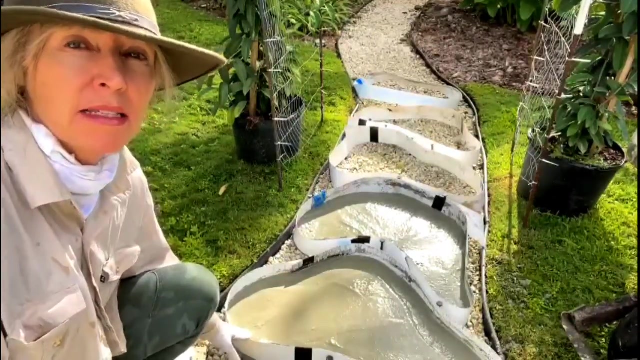 We're adding the second bag. This will allow me to do at least two at a time. This is the perfect time to do a project like this. It's early morning and the sun is just coming out. It's kind of cool right now And it's gonna dry quite nicely. This first one took about 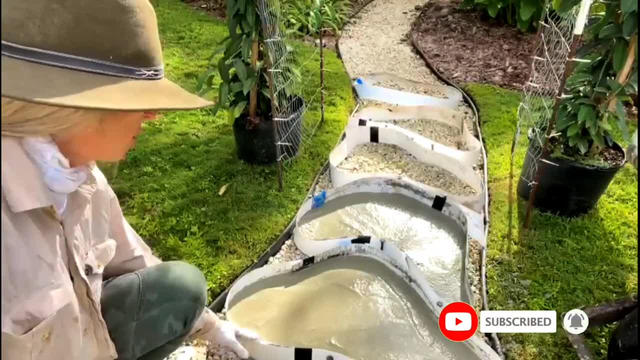 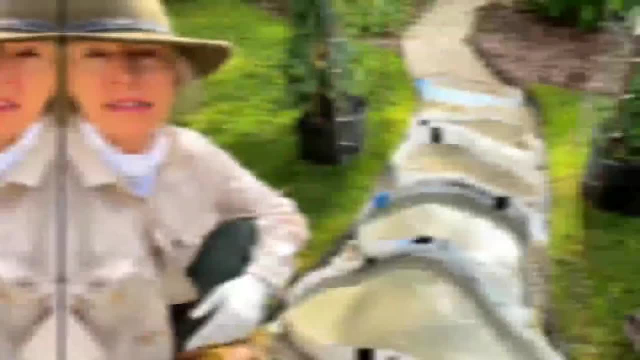 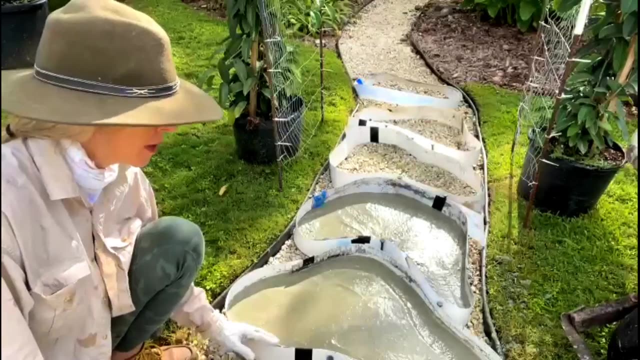 one and a half bags, And I'm building it up to the black liners right here that are guiding the pathway. So we'll let this set for- oh, maybe, I don't know- maybe five, ten minutes or so, Not a long time, And then the forms are removed and as well as the stakes, And then we'll continue on the pathway. 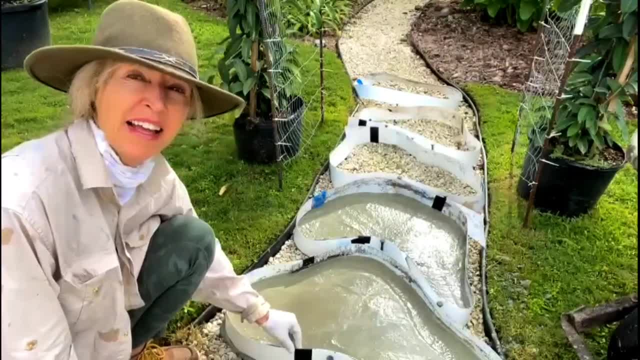 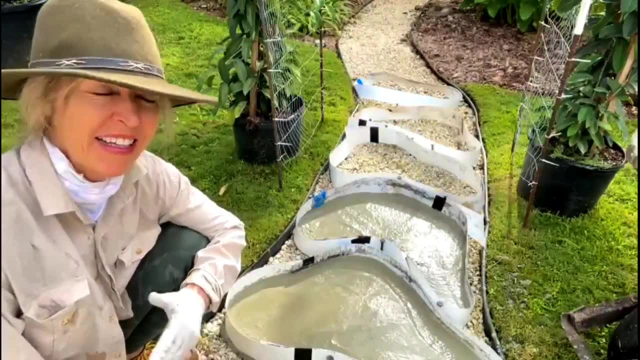 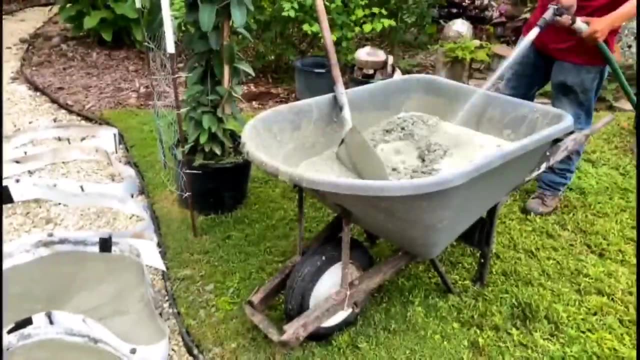 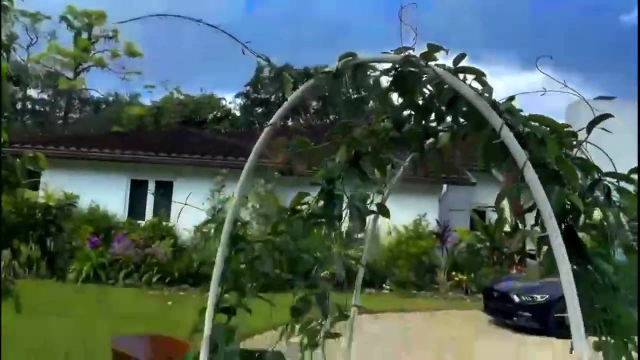 with more forms. It's that easy. You can tell if the forms are ready when you lift up the forms slightly and the concrete doesn't really move. So that's a good sign. And then it started to rain Here. I thought the weather was just so amazing, And it is. 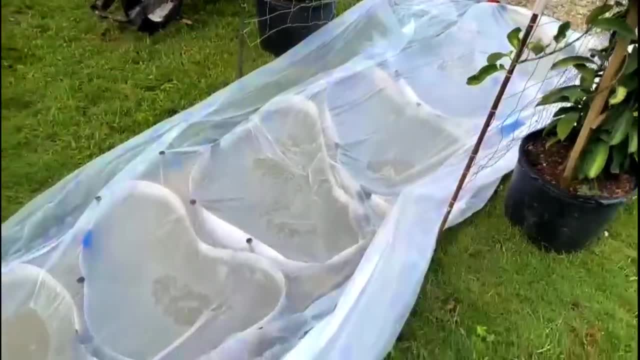 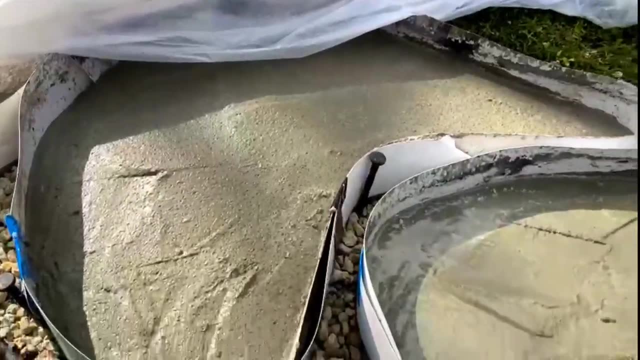 But rain and our concrete really don't go well hand in hand, Especially when the concrete still has to cure. So we just covered it with plastic and waited it out, All right. so it's nothing but a little sun shower And we're going to start removing the forms here. 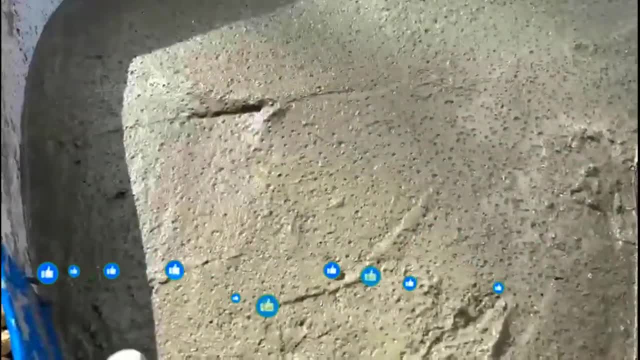 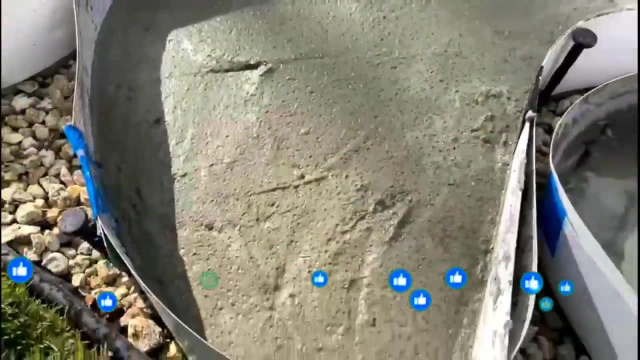 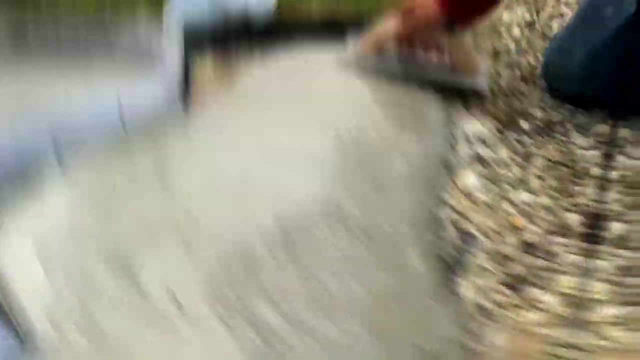 But, as you can see, the rain before we got the plastic on it did leave a few little pebbly-like traces, Like it's a design. It's kind of cool actually, But I don't want it on this And we're going to go and smooth it out again. It becomes a little bit rough on the side right here All. 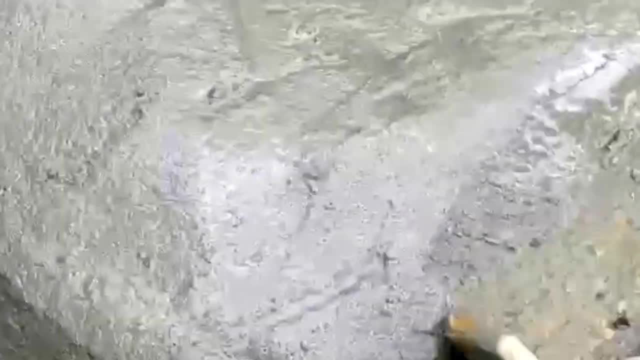 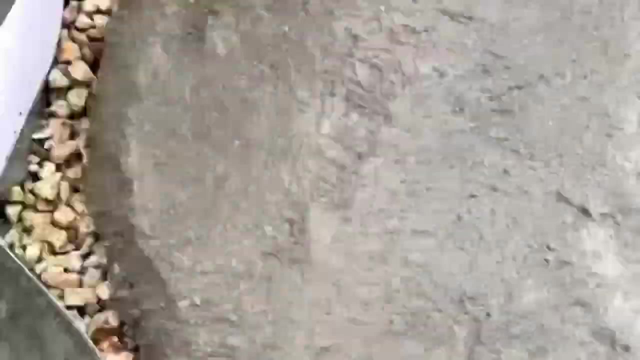 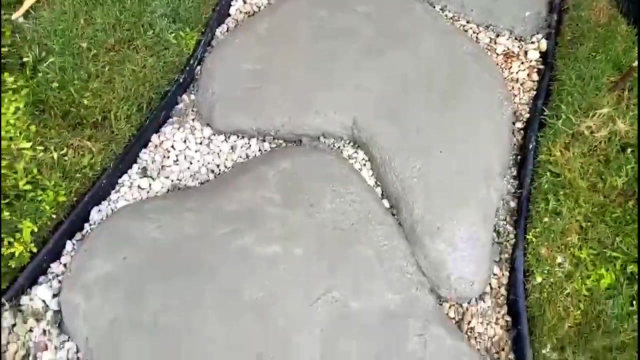 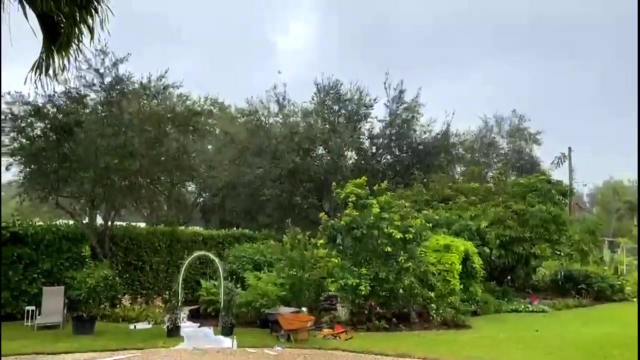 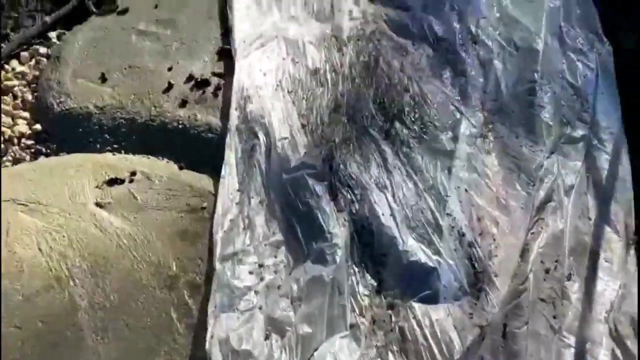 you want to do is take a chip brush like this and brush it down like so, And it rains again. It rained out hard last night and yesterday It poured all day. I'm going to take this off and let these kind of dry out. 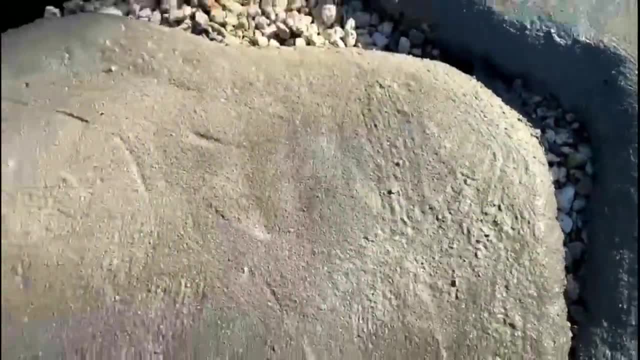 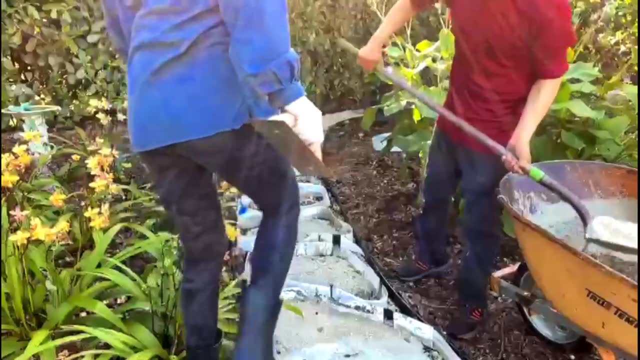 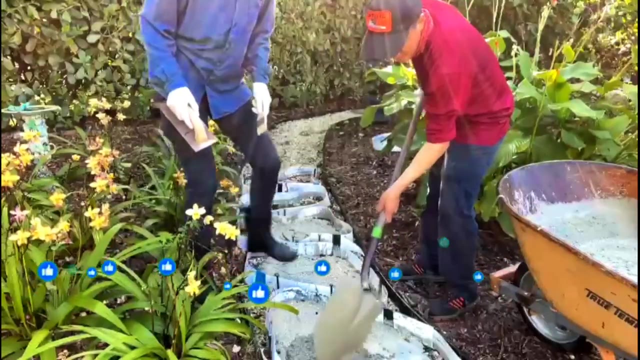 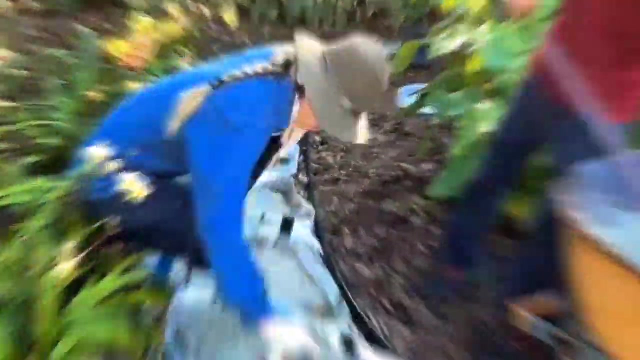 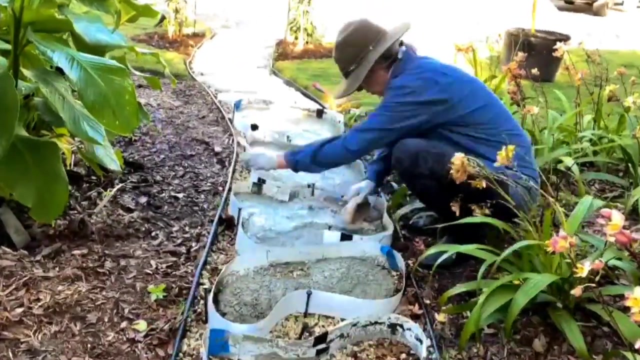 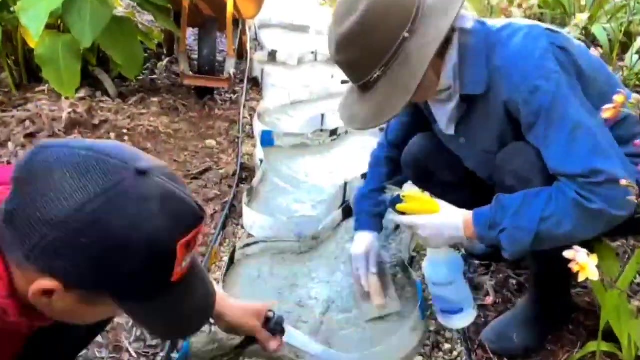 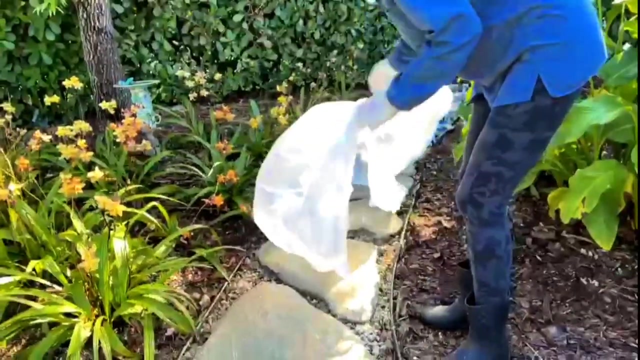 This is really nice, though Look at that. That's hard, It's nice. Wow, We're going to start right here. Fill her up. I'm gonna lay this tarp over- now it's about eight o'clock in the morning, just helps keep. 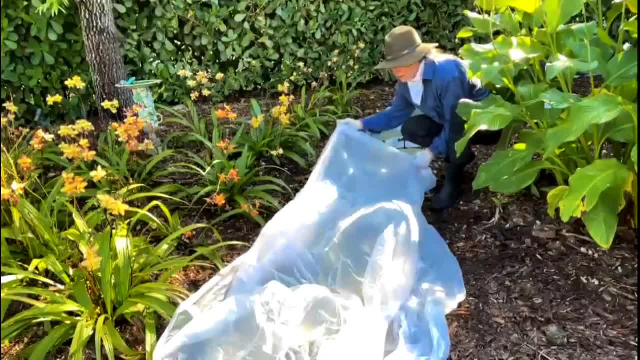 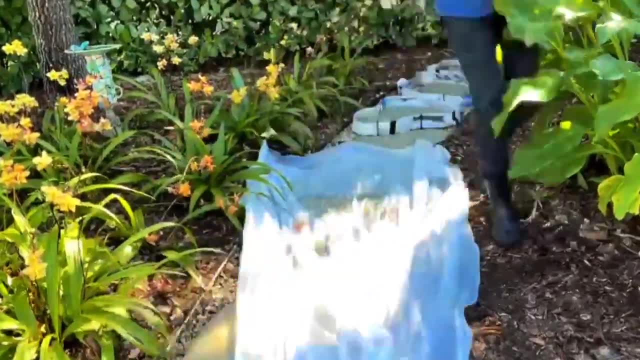 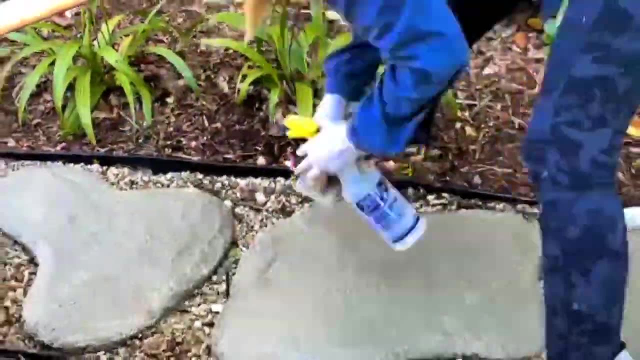 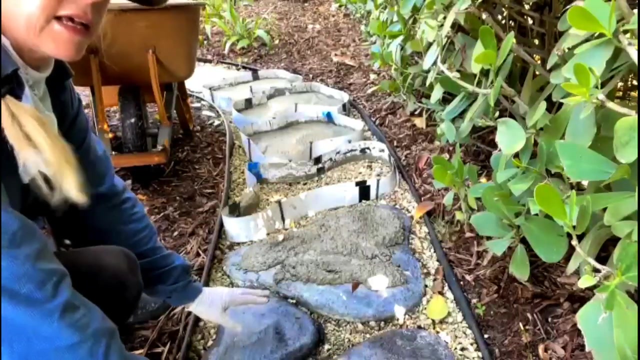 the debris off the concrete and it also just kind of helps it set undisturbed. so here you notice that I colored these like a charcoal color after I had set the stones and it really didn't come out great. I wasn't liking the look. so what we're doing now is doing a top. 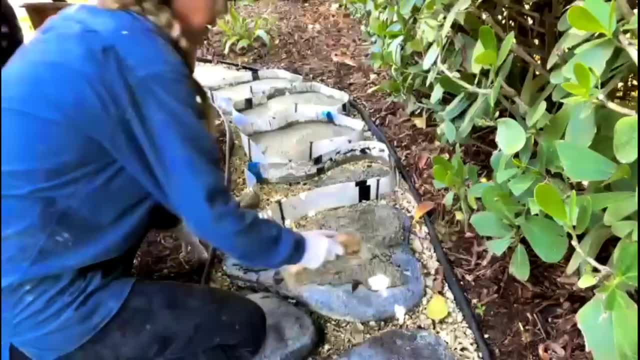 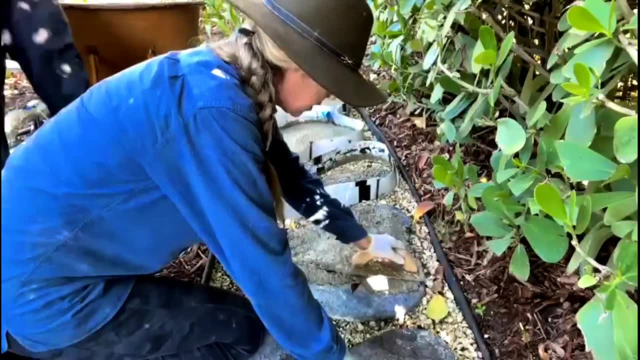 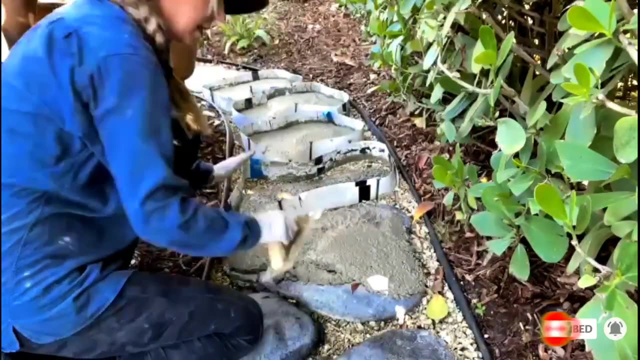 coat of the regular concrete mix that we do all the other stones with and basically just just a top coat, and I think this is gonna be just fine, the coloration that we want. it's looking very organic, the color and as well as the shape, so I'm not resetting the form around the piece. I mean you could do that, but you really want you to in this case. 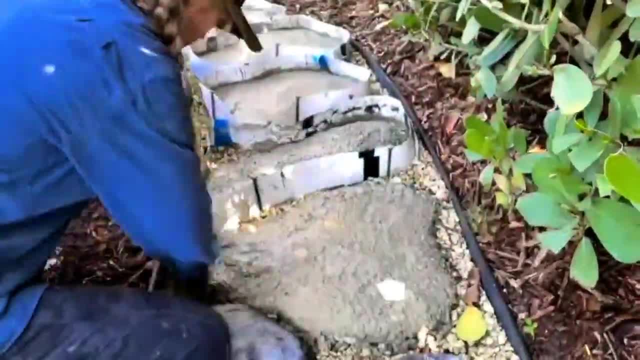 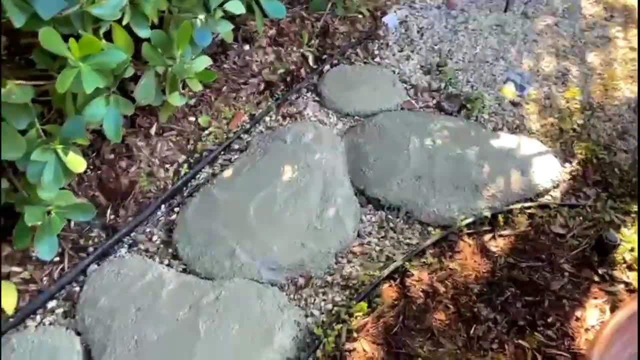 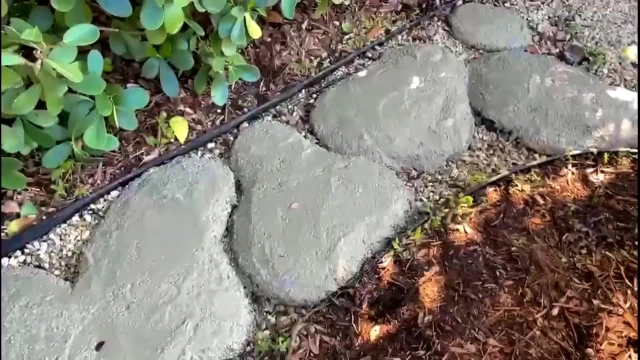 we made it to the end of the pathway. this, as you put the call, was where I had colored the concrete stones a charcoal and I didn't like it. I didn't much care for it, so I changed it up and now we're going to do the top coat of the regular concrete mix that we did earlier. 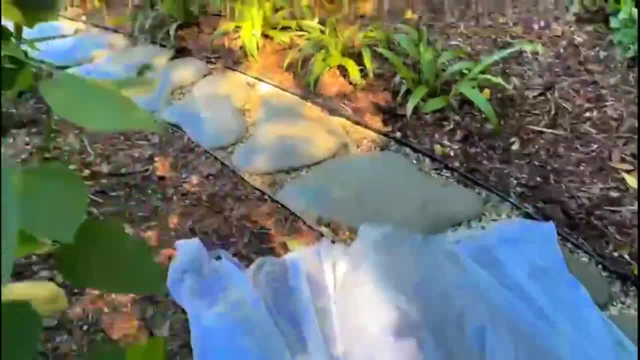 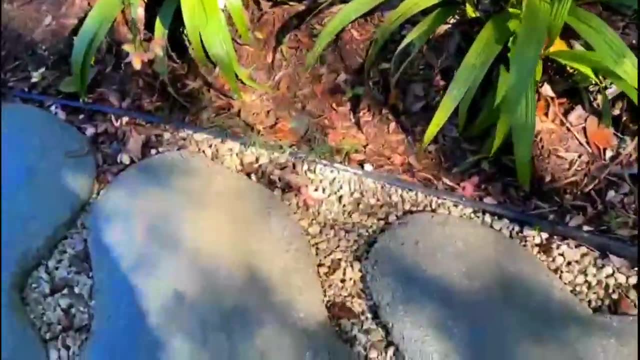 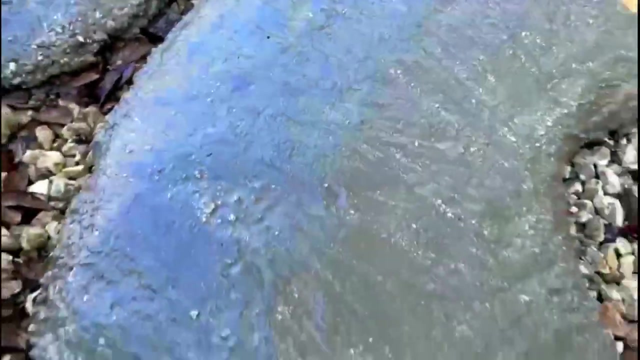 we're just simply taking the plastic which we had put over the top of the stones back here and we're taking them and making these little imprints. I'm going to show you real close to see if you can see that. let me see, see those little imprints there. I love that texture and that is created by plastic. 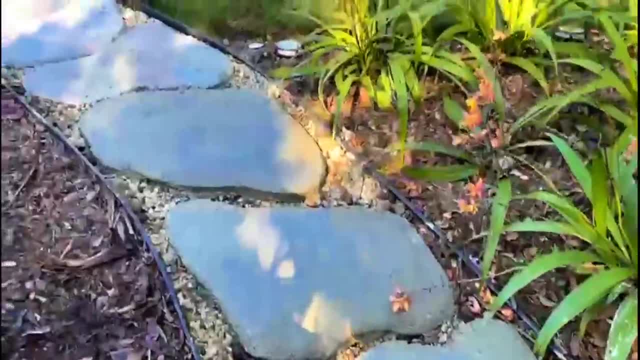 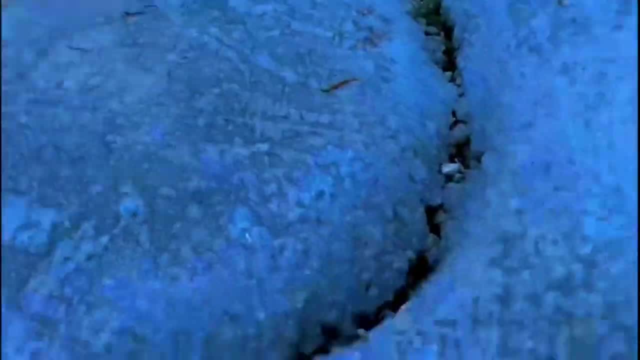 now you can actually put the plastic on and leave it to dry, like we did over here, and we did this just because it started to rain out and you can see the color is a little bit lighter than the ready. let me see if I can get. there's a lot of shadows here. let me see if I can- okay, see that. 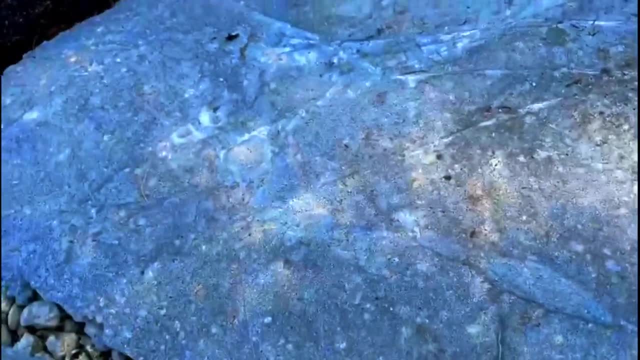 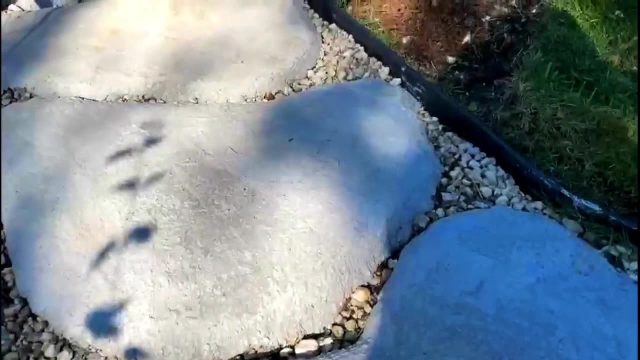 texture. I happen to think that's really pretty. if you don't want that in there, of course you don't have to have that in there, but that was done by laying in the plastic. when it started to pour out, we just laid the plastic over it to prevent, uh, the the concrete from getting destroyed by the. 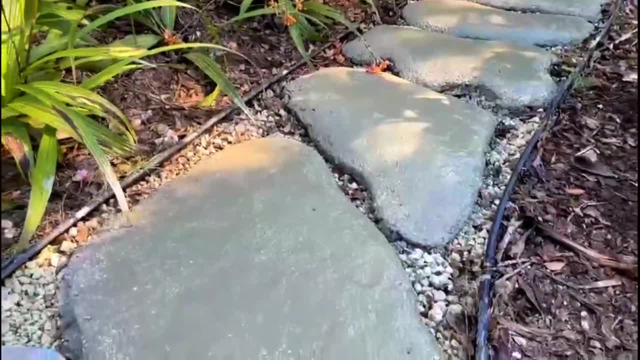 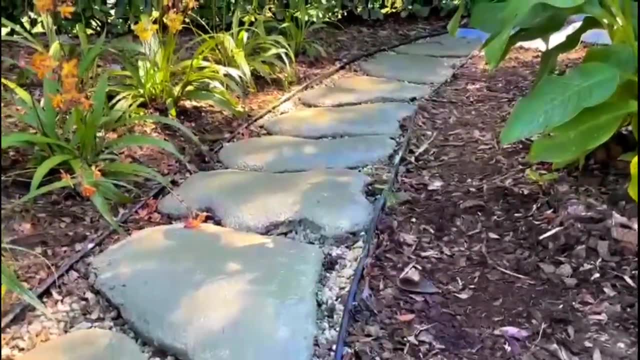 pouring rain, and that is why, actually, it's taken so long for me to finish this project, because there's been so much rain here, and that's okay. um, right now we're gonna complete the rest of this and I'm so excited. I can't wait to show you the reveal. 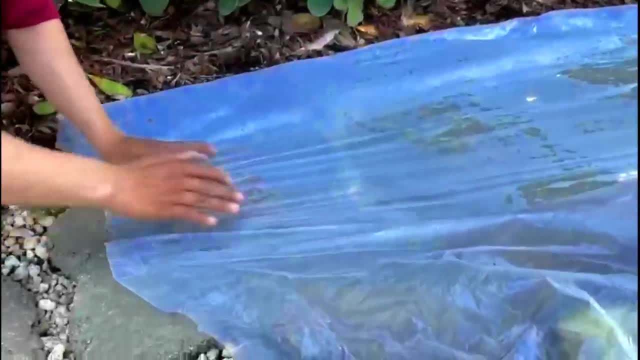 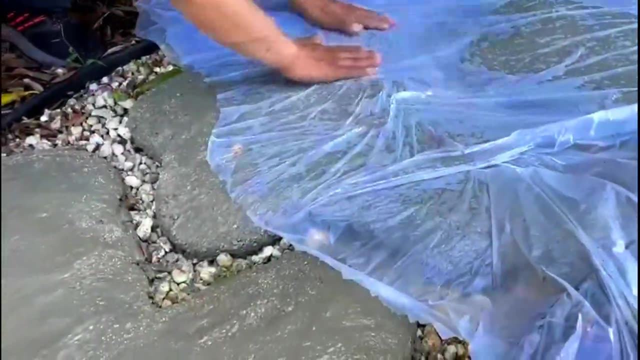 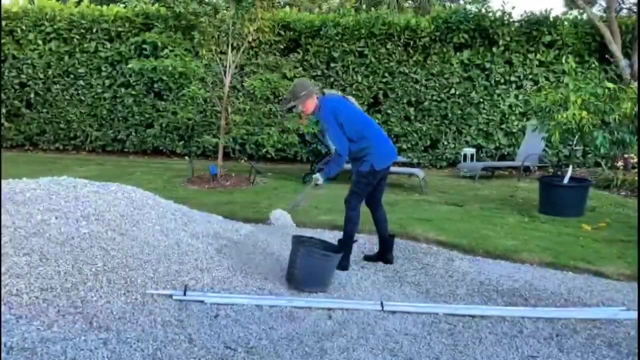 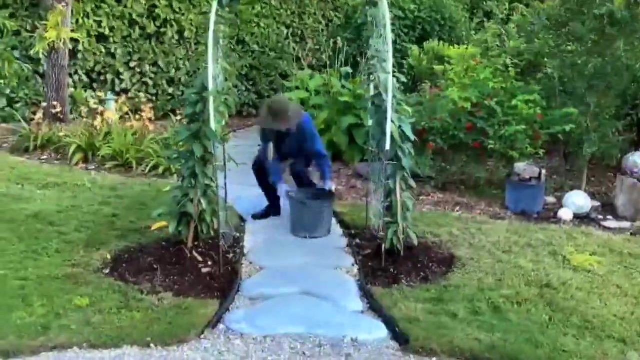 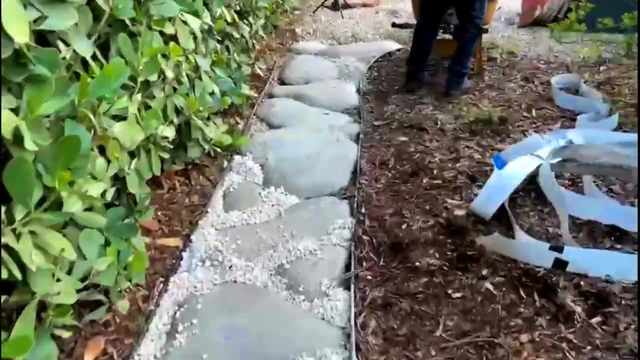 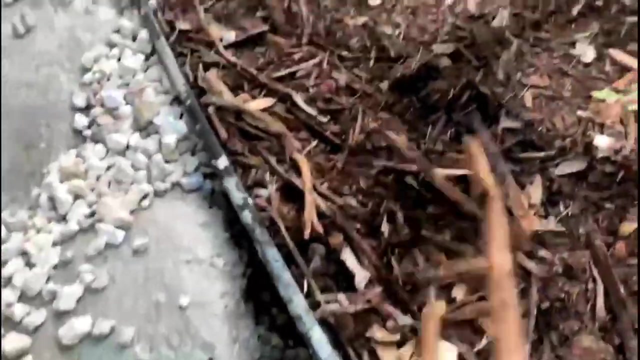 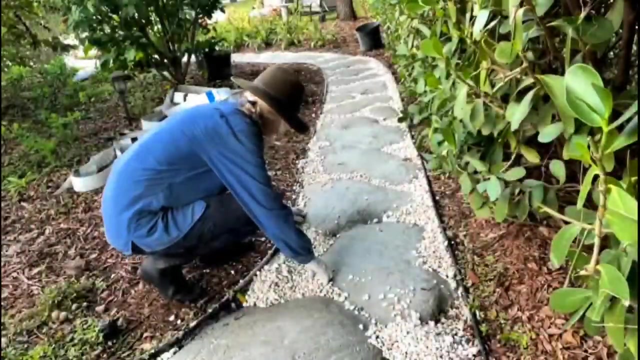 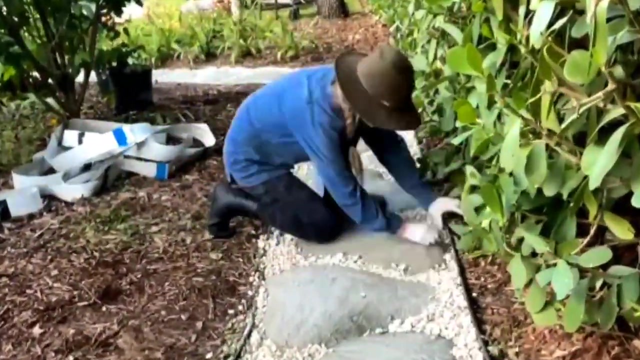 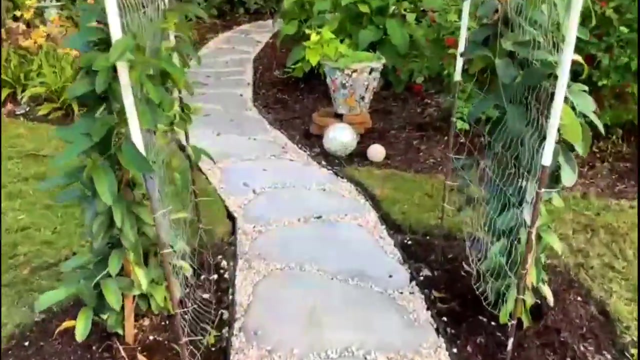 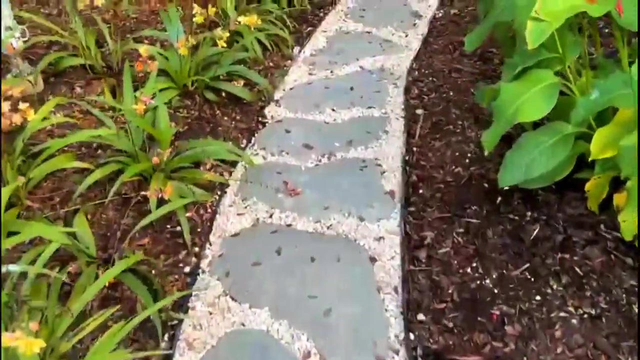 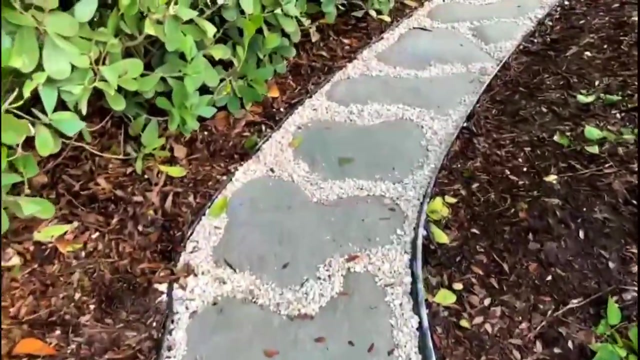 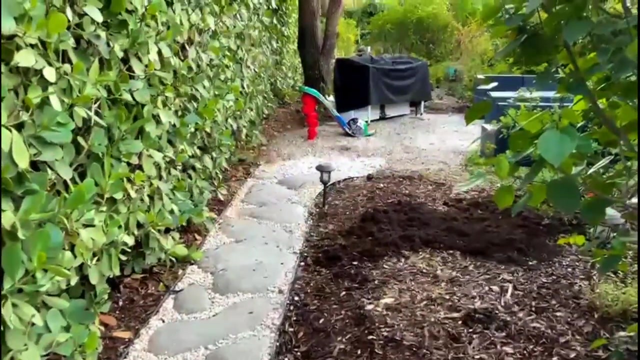 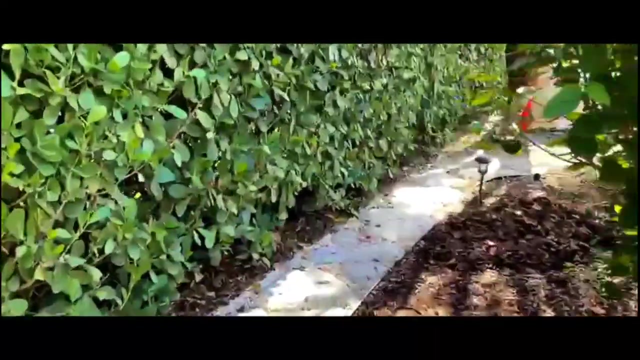 I can't wait to see the reveal. What am I saying? That plastic creates such an organic look. It's so pretty to manipulate the concrete like that. I can't wait to see the reveal. I can't wait to see the reveal. 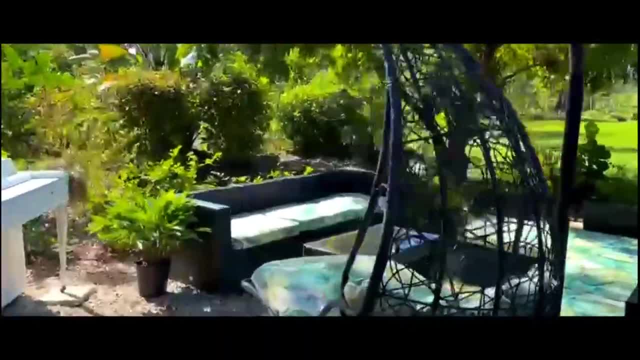 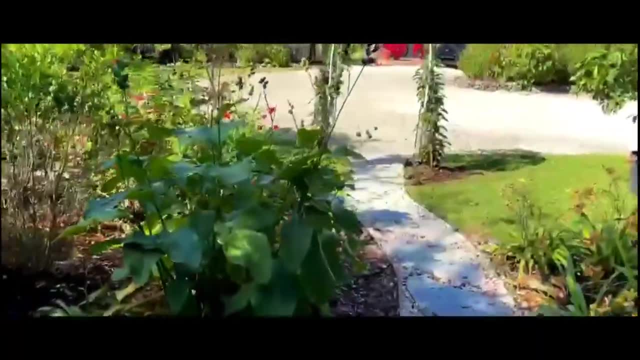 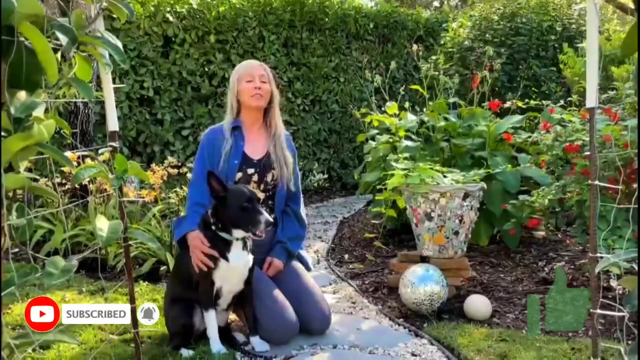 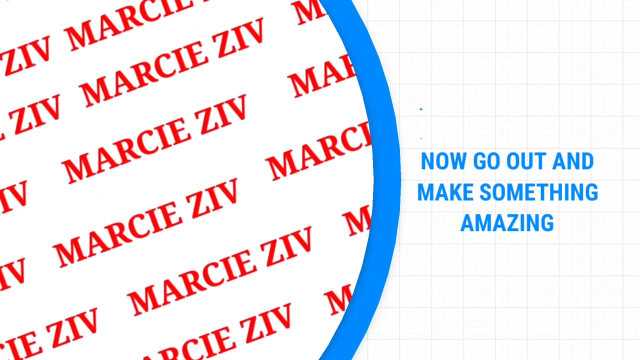 I can't wait to see the reveal.